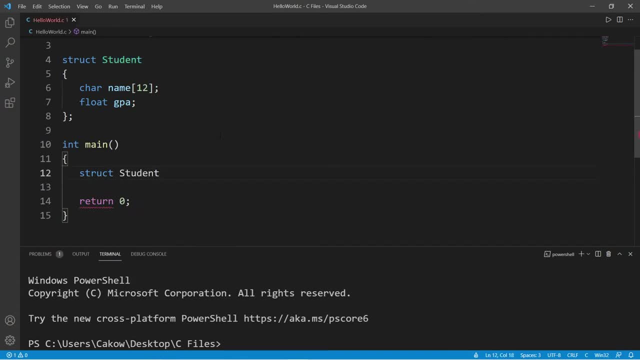 type struct, followed by the tag name and then some variable name to identify each struct. So let's say we will have four students overall And I'll go ahead and assign some values right away when we initialize this struct. So we need a name and a GPA. So the first student. 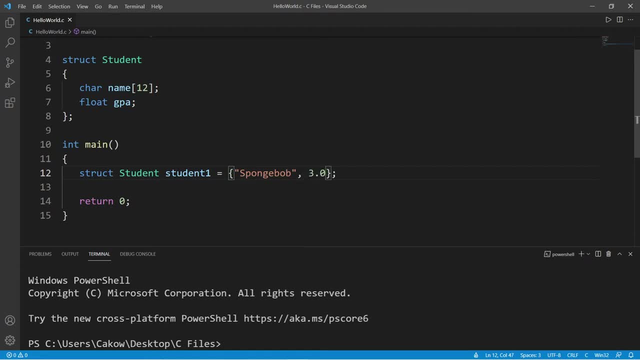 let's say, is Spongebob, And Spongebob has a GPA of 3.0. So we can copy this and paste and create a few more students. So student one, student two, student three and student four. Next we have Patrick. Patrick has a 2.5.. Then Sandy. Sandy is smart, so she has. 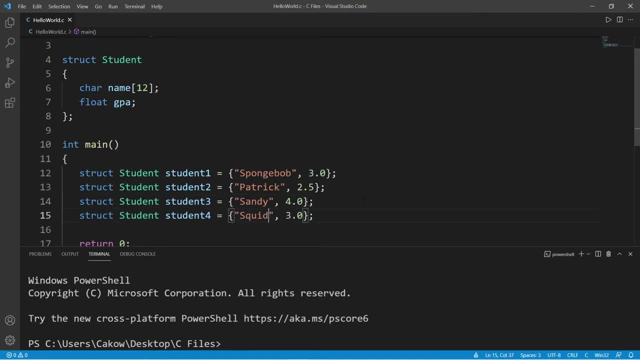 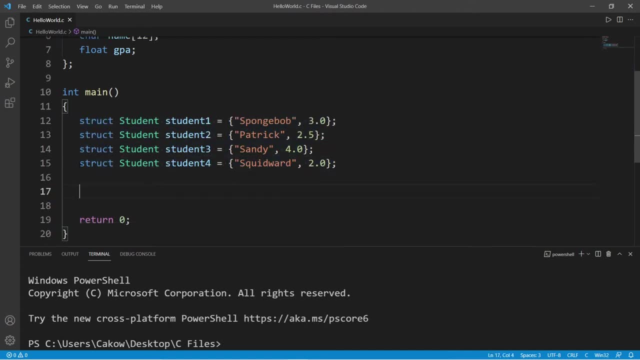 a 4.0. And Squidward Squidward has a 2.0. So we have four students. Now we will create an array, So the data type of our array, what it's containing, will be structs. It will. 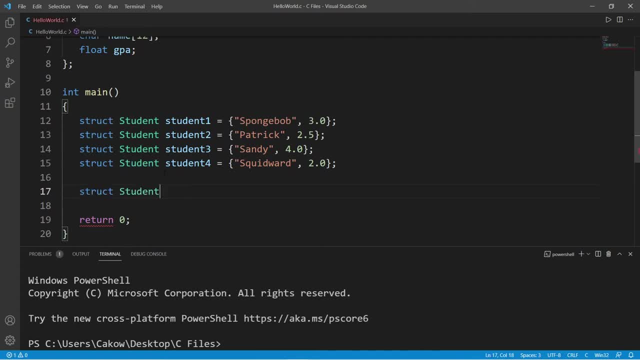 be struct student. It's kind of like the data type. So with an array you have to declare what you're going to be putting within the array- struct students- and then we need an array name. So this will be students, And then specify a maximum size if you need one. 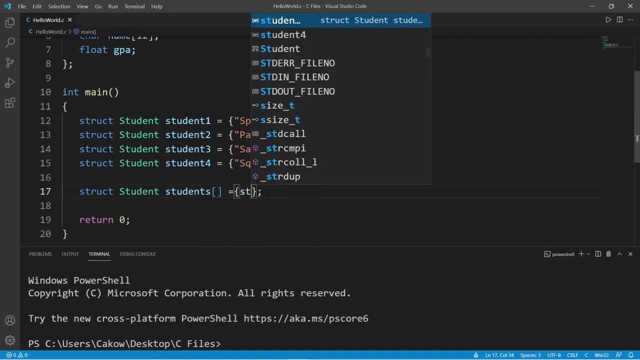 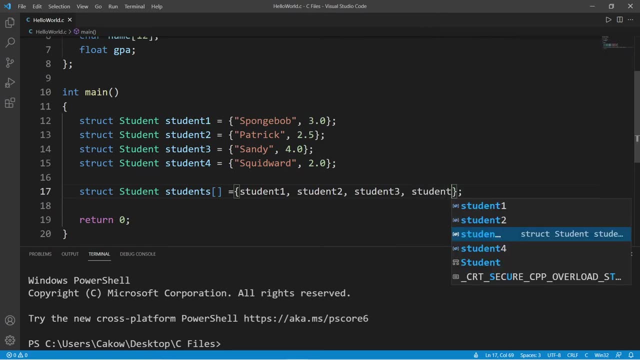 But I'm just going to initialize this array with some students. So let's add student one, student two, student three and student four, And there we go. We have an array of structs. Now, if I would like to display each of these structs, 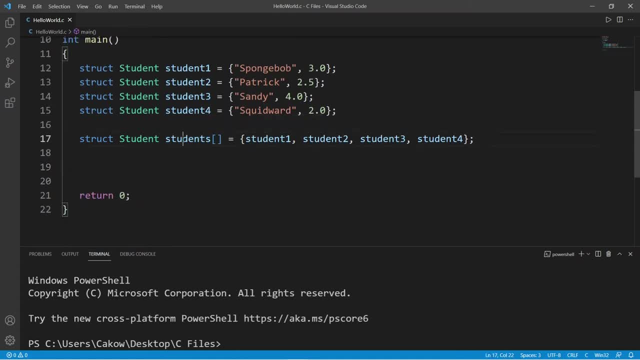 Now, if I would like to display each of these structs student's name, I can use a for loop to loop through our array. So for curly braces, we will create an index int. i set this equal to zero. we will loop through this as long as i is less than. 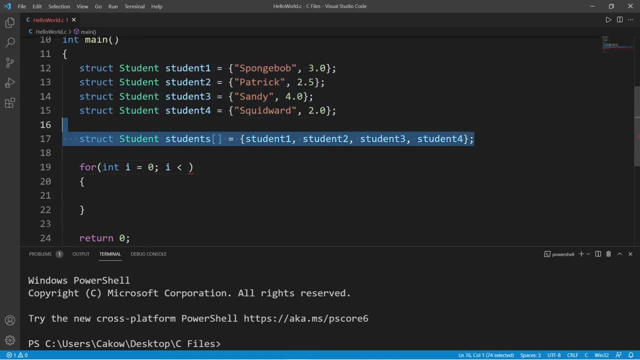 and then we need to calculate how many elements are within our array. So we have four elements, but we can do that by using the size of operator pass in our array and then divide this by the size of one of these elements- Size of students- and then pick maybe the first element of zero.